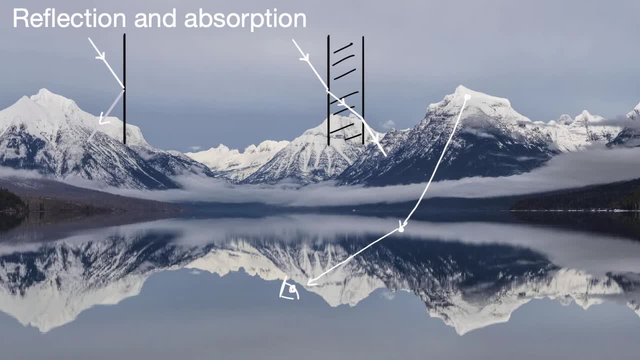 and doesn't transmit any through it if it's completely absorbing, And so that would be a situation like this. Now, the reality in the real world is we have oftentimes a little bit of all of the above happening, For example, when we look at this white snow up here. 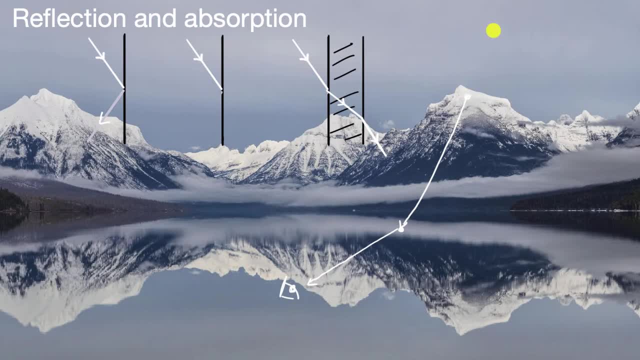 this is reflecting pretty well. So there's light that's coming from the sun, or maybe it's being reflected off the clouds, or maybe it's getting through the clouds and when it hits that snow, it gets reflected. Now, the reason why we don't see a reflection: 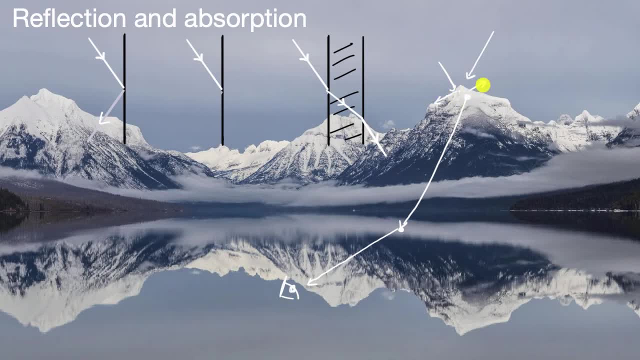 the way that we see in this lake right over here is the snow reflects it in all different directions, But the fact that it's that bright color- in fact, you might need sunglasses to look at the snow just as much as you need to look at the sky- 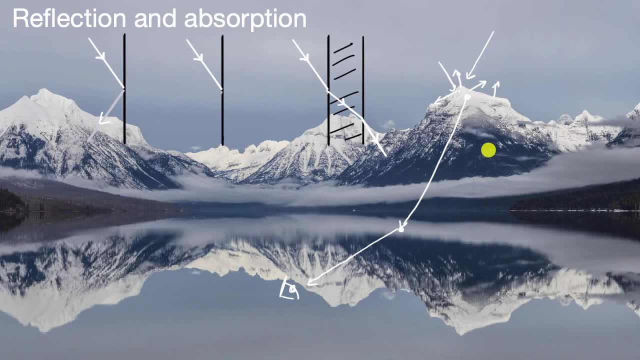 is that it's reflecting most of the light. But if you go down here, where we see the trees, the same light from the sky is hitting it, but not as much light is coming back to our eye, And that's because this part of the mountain. 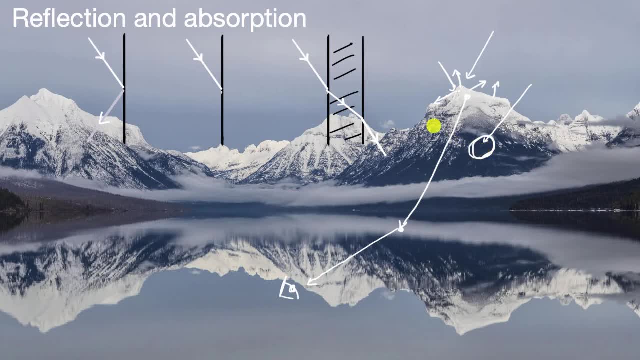 it might be trees, it might be rock, it might be dirt- is absorbing more of the light, But it's still reflecting some. We can still see it a little bit. So this might be where most of it is getting absorbed, but a little bit of the light gets reflected. 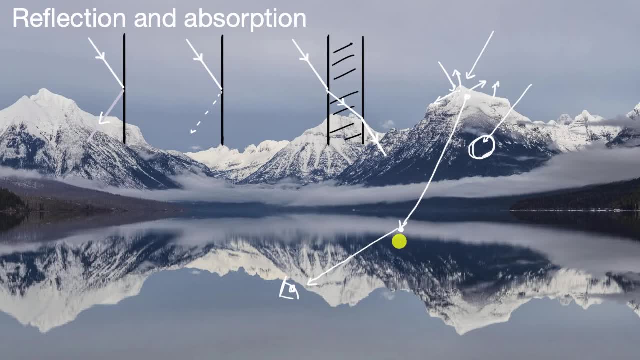 which we can see right over there And if we think about the water right over here, some of the light is probably making it through and probably refracting as it does, so Some of it is getting absorbed as it makes its way through the water. 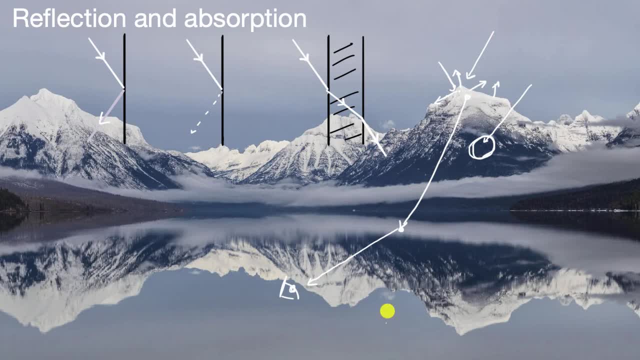 If this was a really deep lake, when you get to the bottom it could be very, very dark And then, as we talked about, it looks like a good bit is reflecting When we look at the image that we see in the lake. 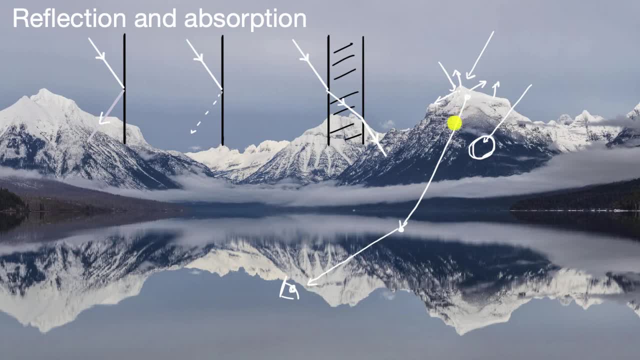 it looks almost as bright as the real thing. So, as I said, this is happening all around you. In fact, when people make fancy computer graphics, they actually try to do exactly what the light would do in the real world: to make an image for your eyes. 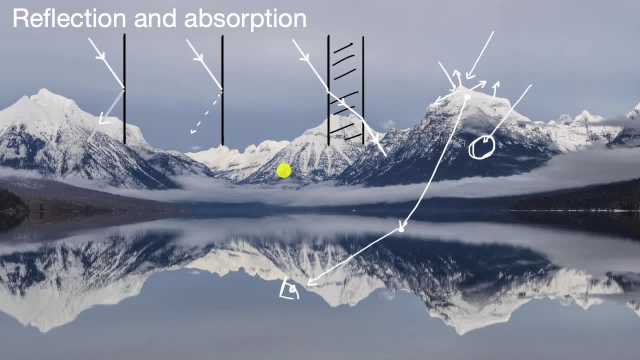 that look like the real world And they're thinking exactly about this: how much gets through substance, how much gets reflected and how much gets absorbed. And, as I mentioned, it's not just light waves that do this. Waves in general can do all of the above.